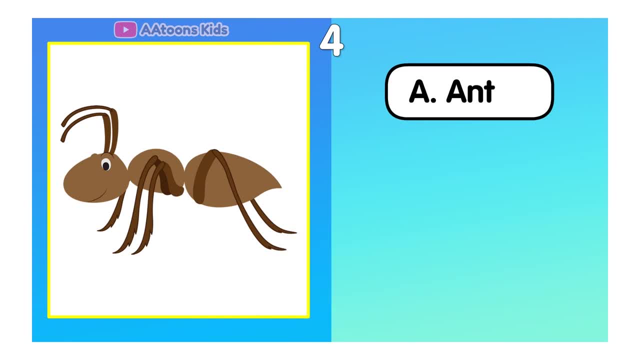 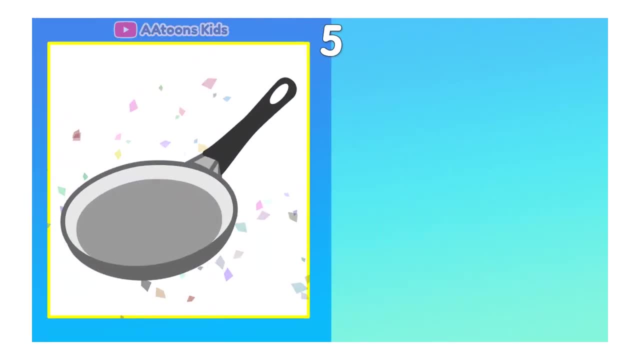 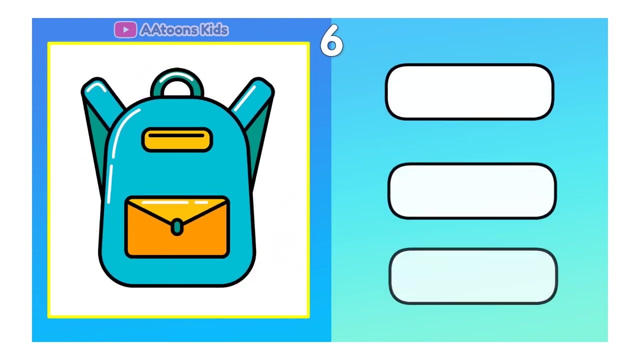 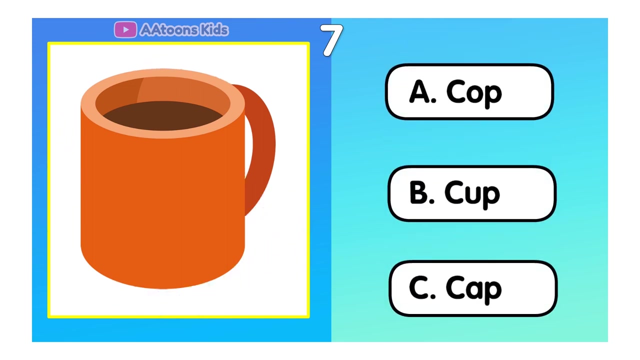 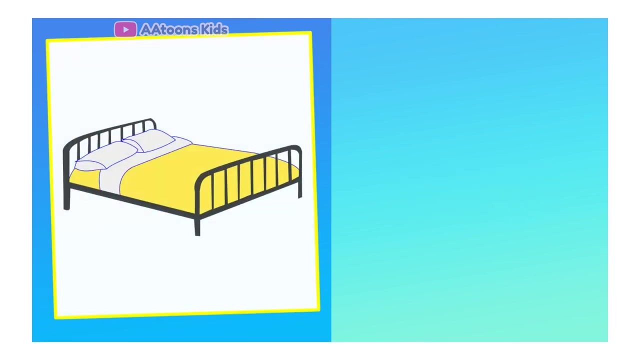 Identify the image and choose the correct spelling. Identify the image and choose the correct spelling. Ant: Identify the image and choose the correct spelling. Pan: Identify the image and choose the correct spelling. Bag: Identify the image and choose the correct spelling. Cup: Identify the image and choose the correct spelling. 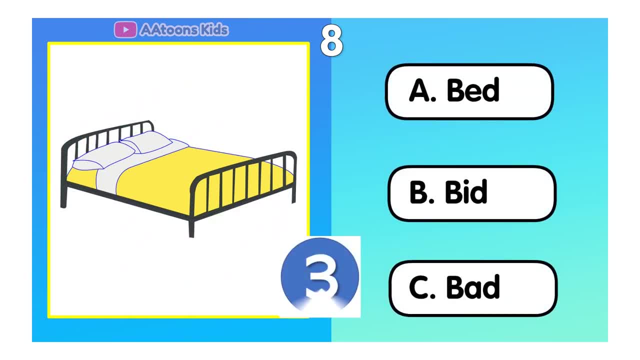 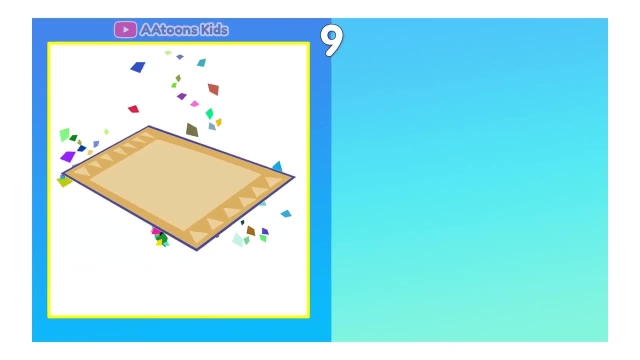 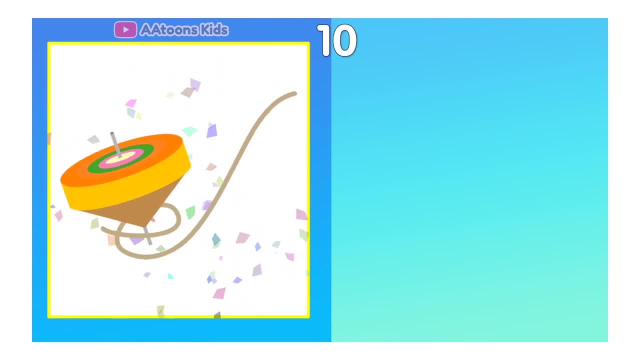 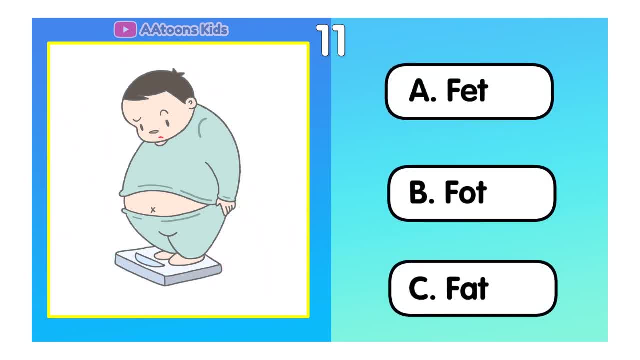 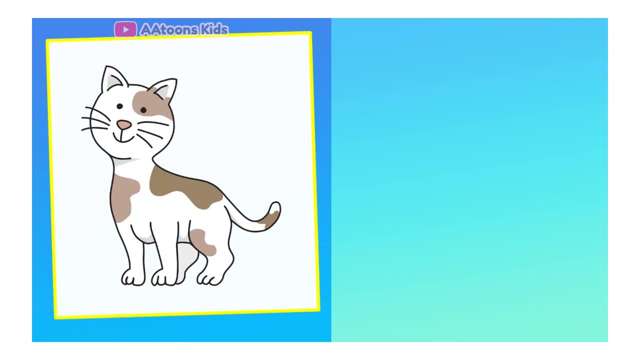 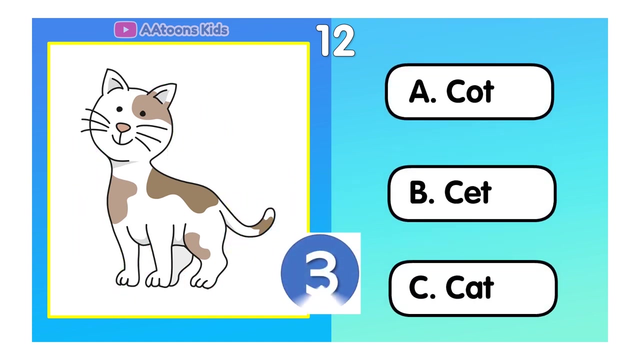 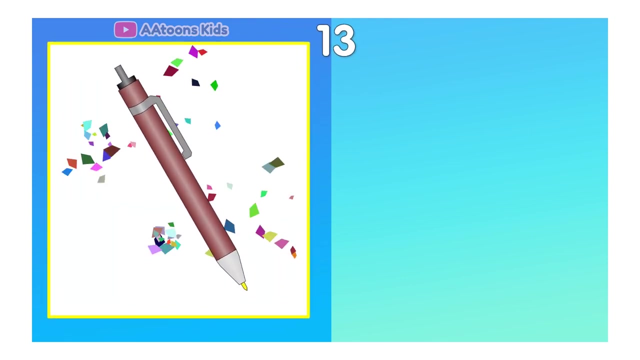 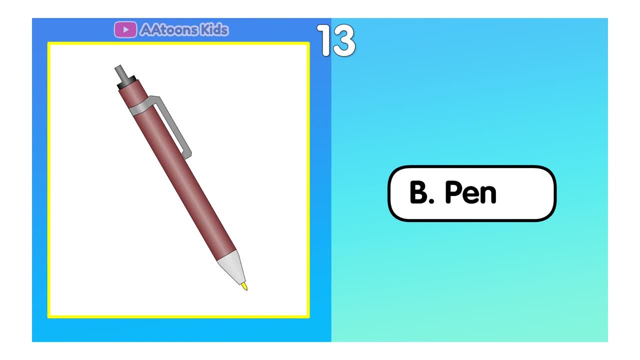 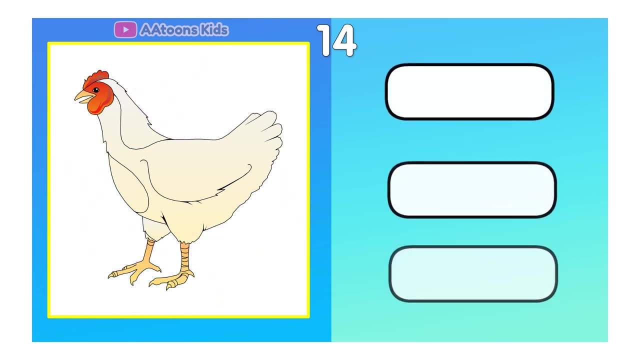 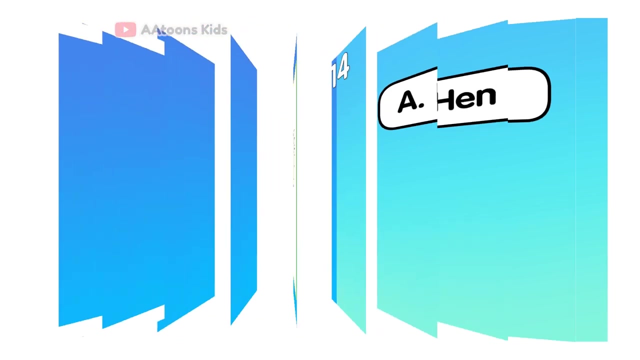 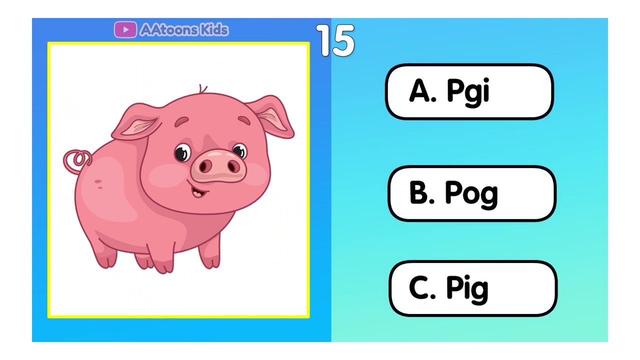 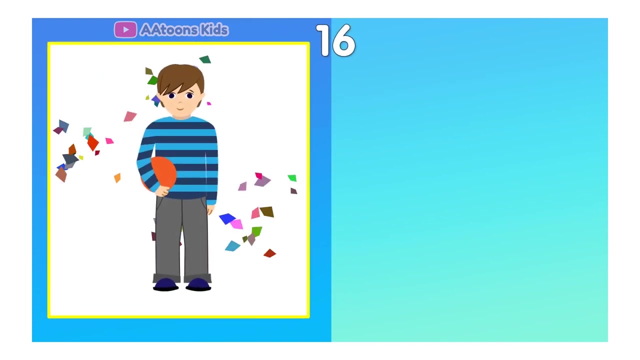 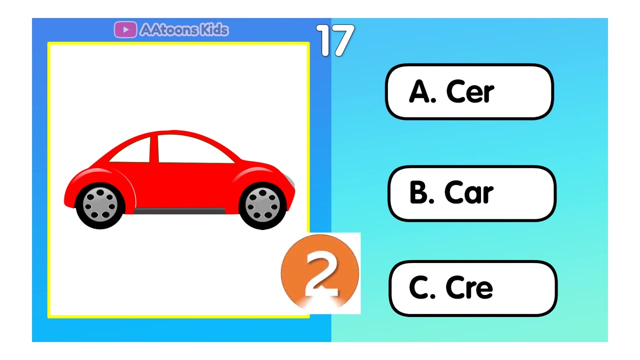 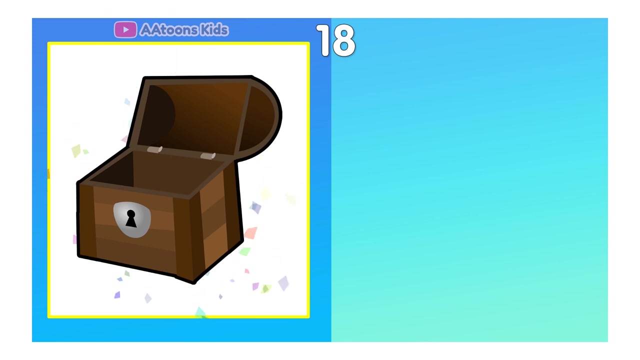 Pain: Identify the image and choose the correct spelling. Pain Pain. Identify the image and choose the correct spelling. Pig: Identify the image and choose the correct spelling. Boy: Identify the image and choose the correct spelling. identify the image and choose the correct spelling. walk: 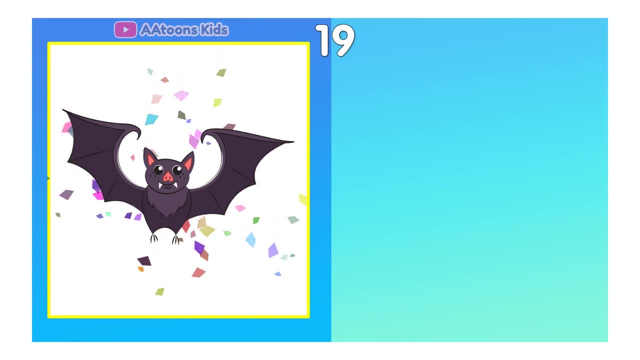 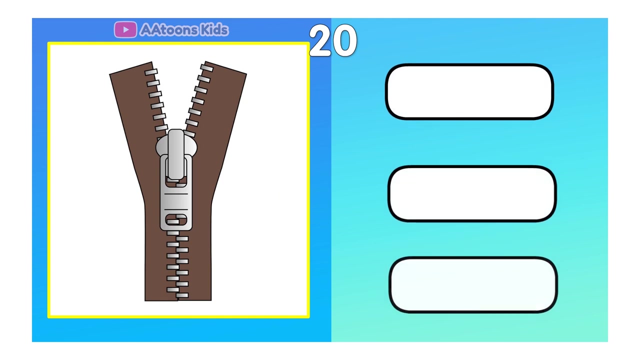 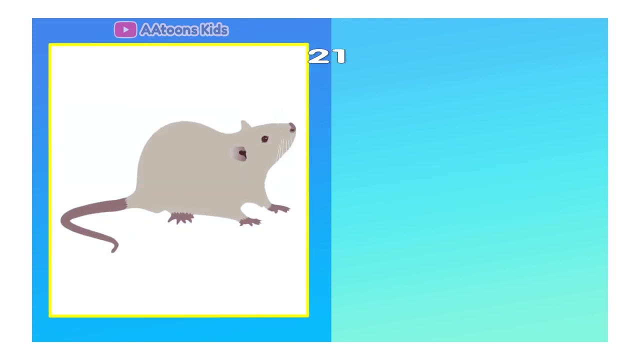 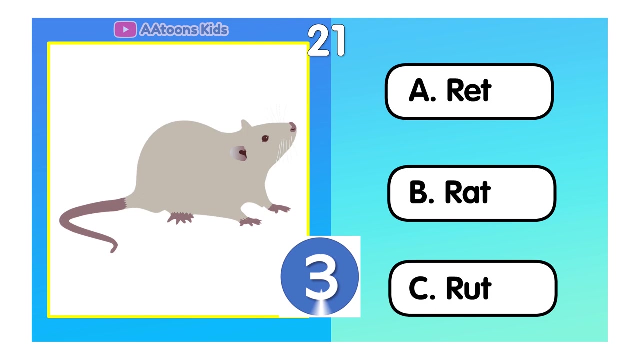 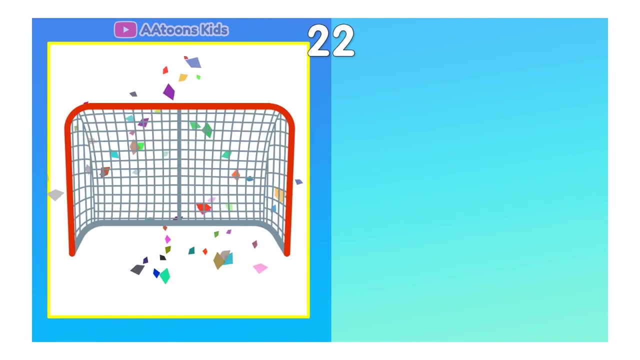 identify the image and choose the correct spelling bath. identify the image and choose the correct spelling jeep. identify the image and choose the correct spelling rat. identify the image and choose the correct spelling rat. identify the image and choose the correct spelling rat. identify the image and choose the correct spelling. 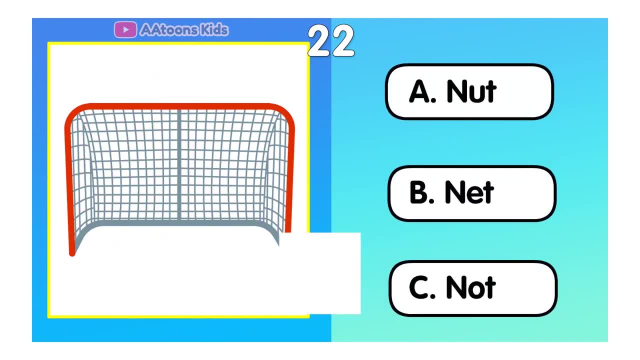 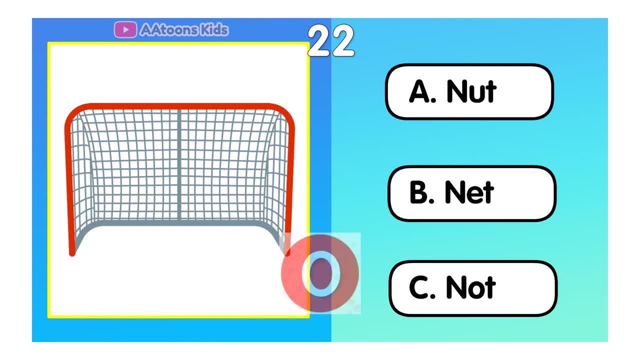 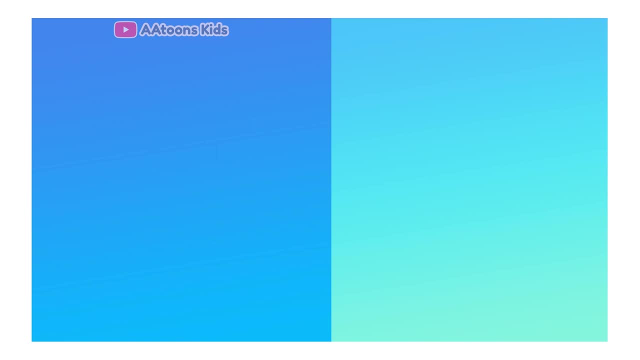 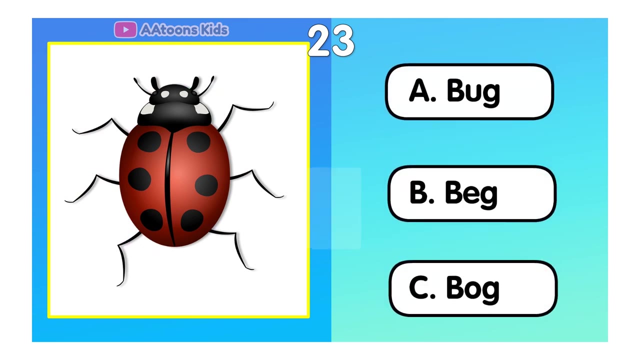 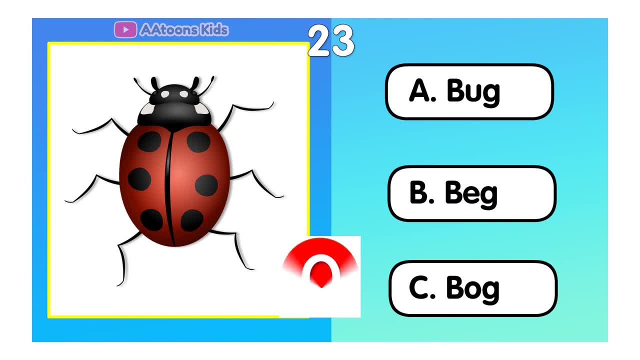 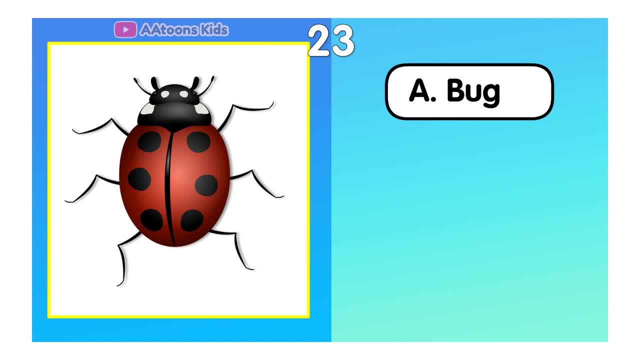 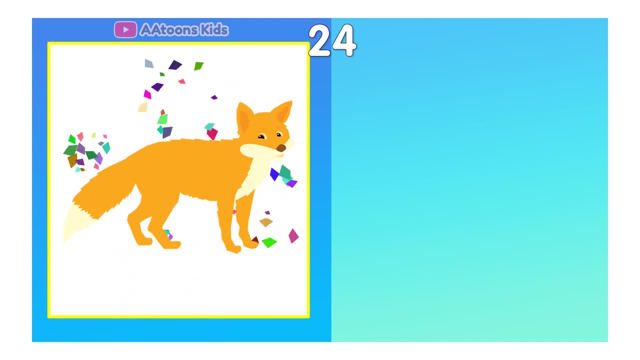 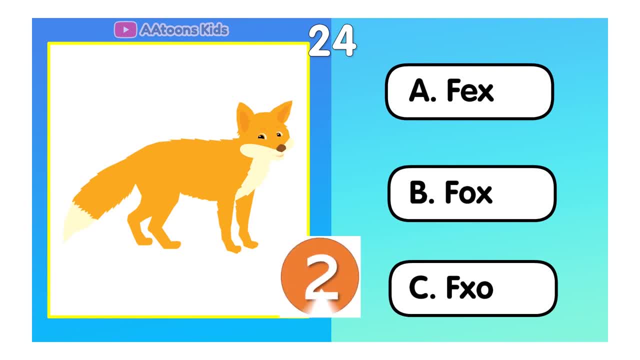 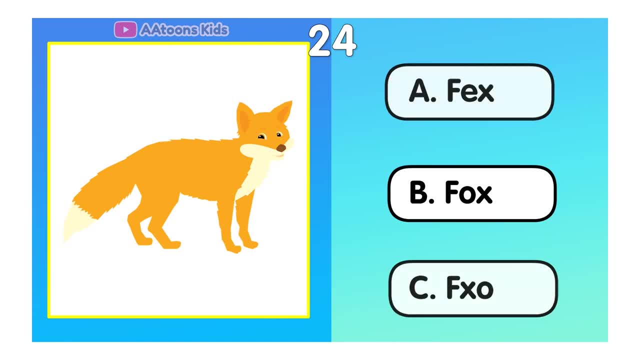 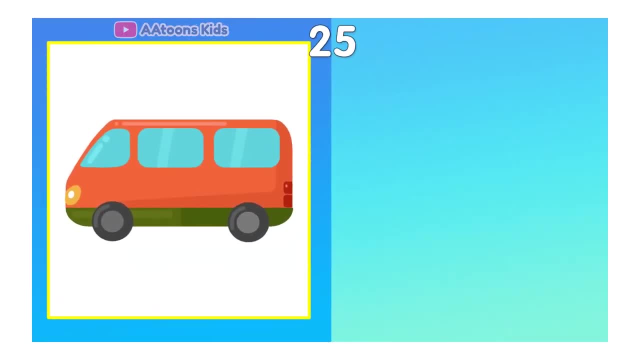 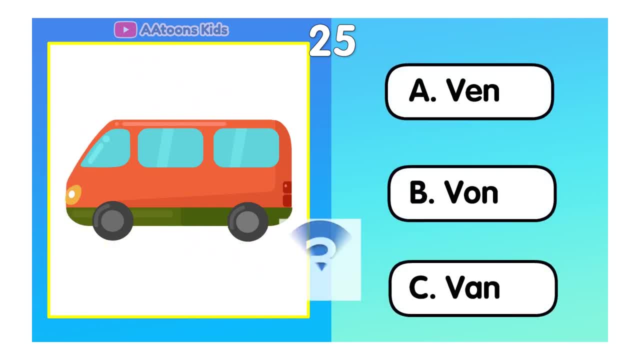 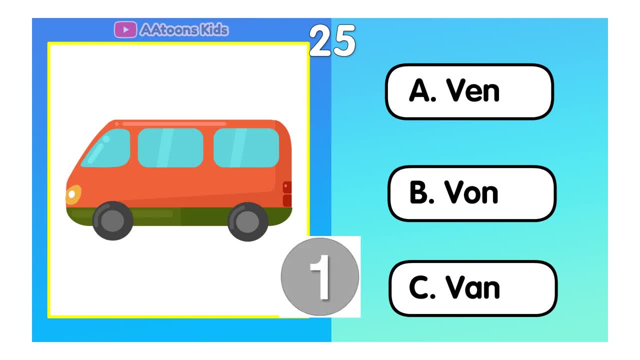 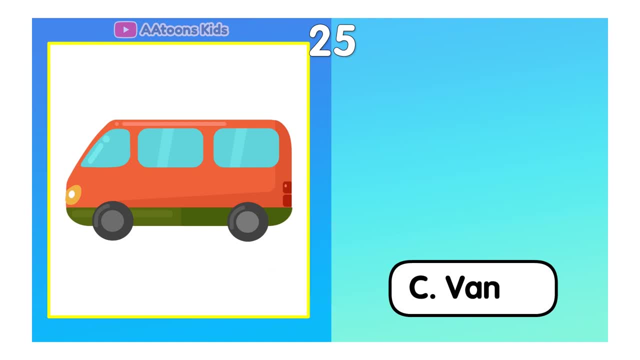 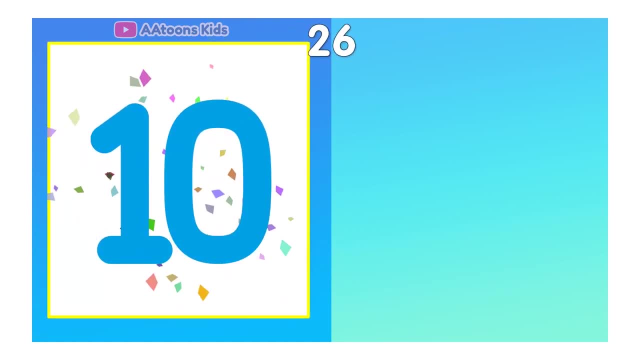 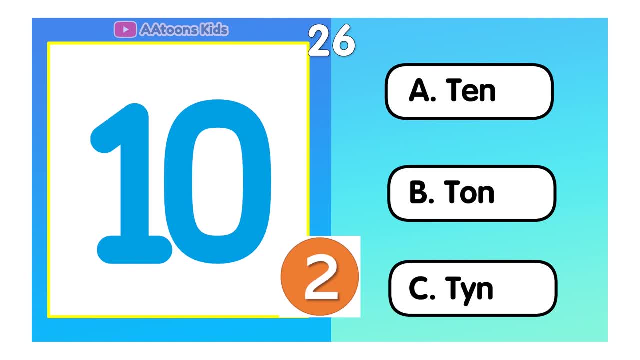 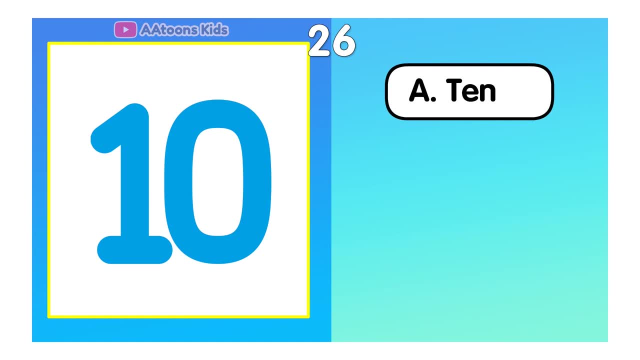 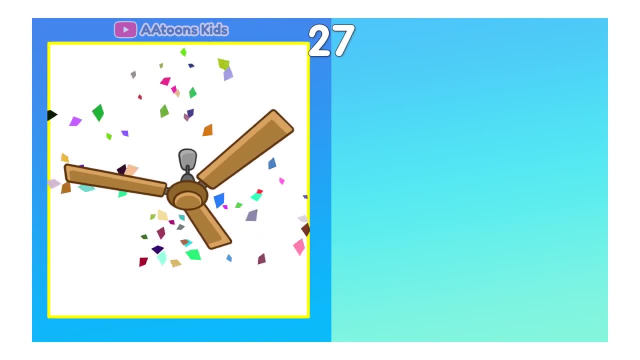 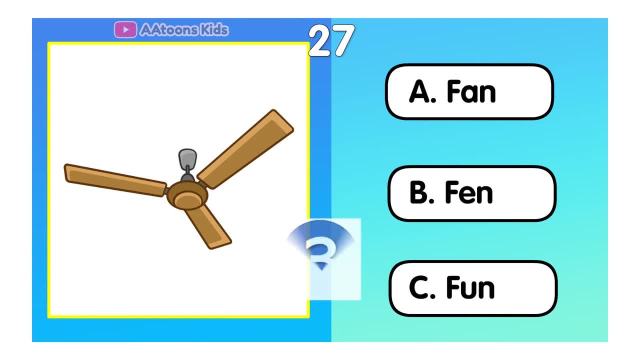 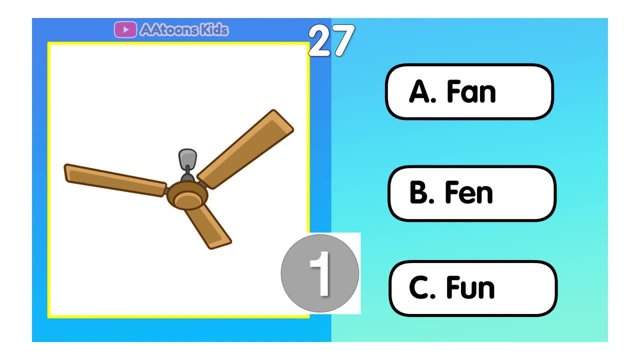 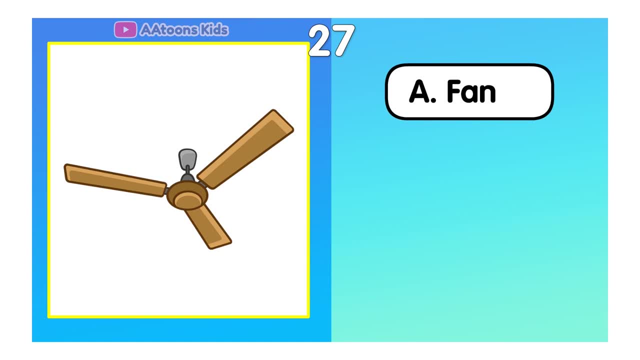 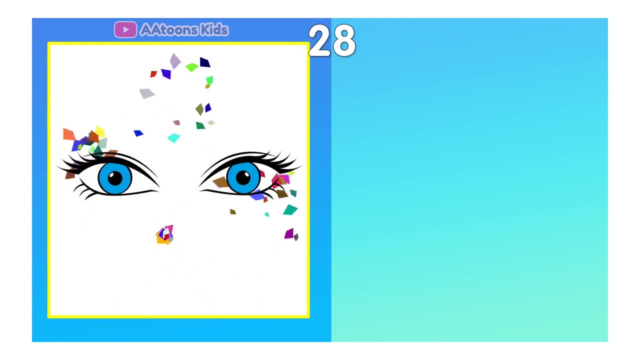 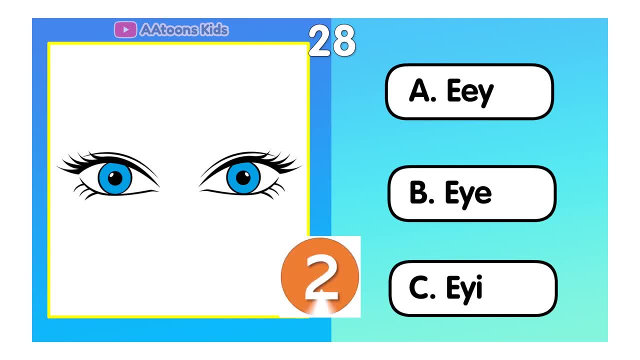 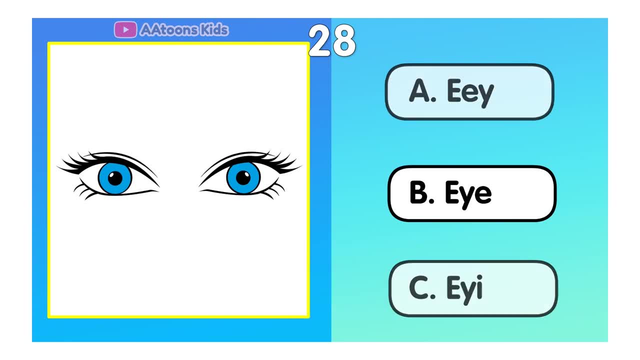 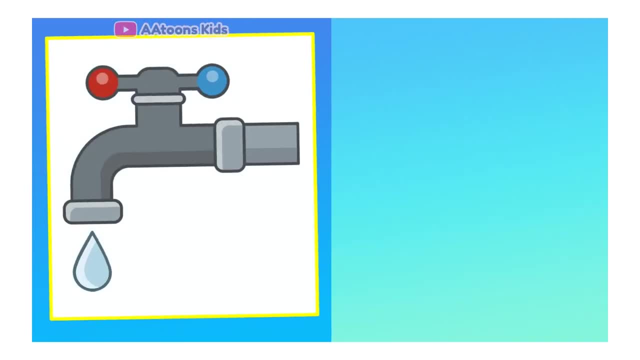 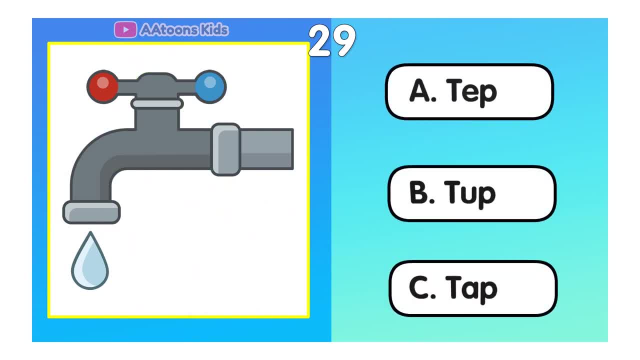 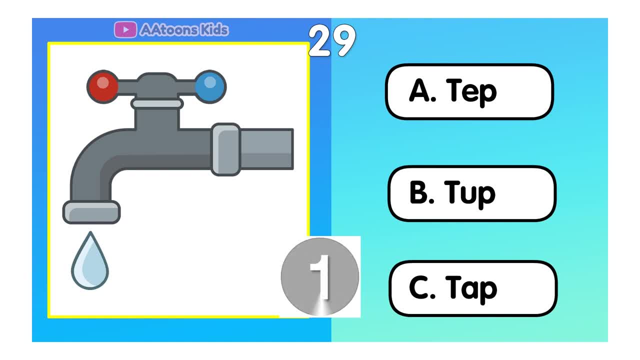 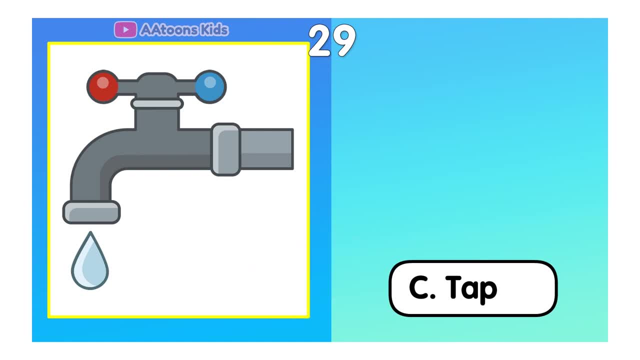 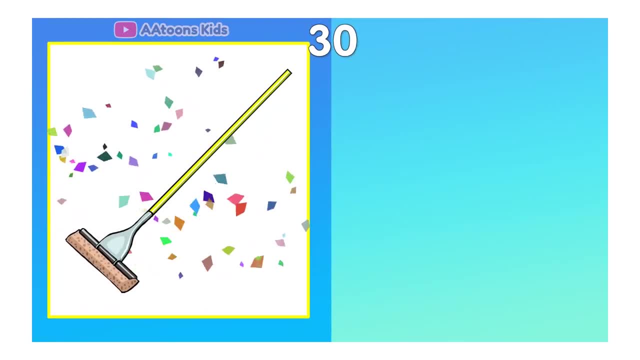